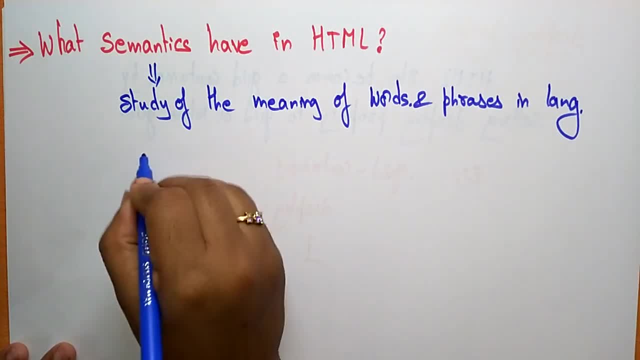 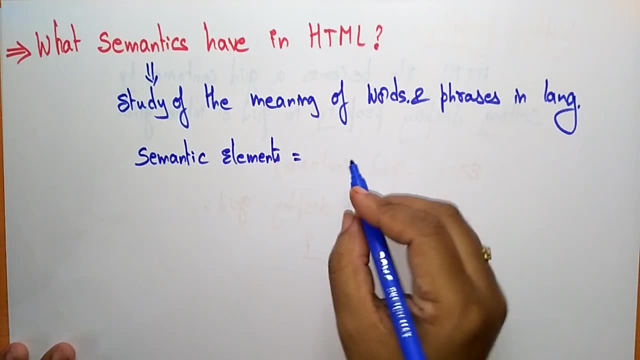 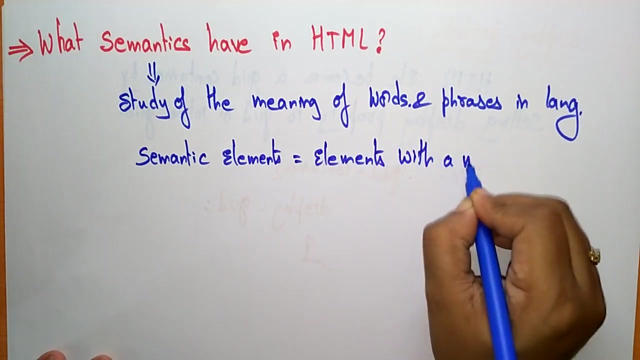 So in HTML you are having the semantic elements. So what that semantic elements? Semantic elements is nothing but elements with a meaning, Elements with a meaning. So whatever the HTML element that you are using, if that element is specifying the meaning of that usage, okay that you call it a meaning. 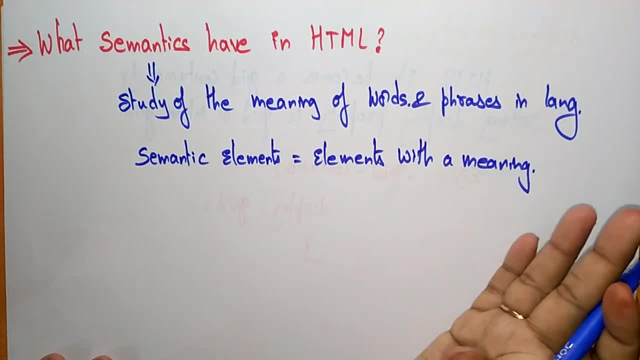 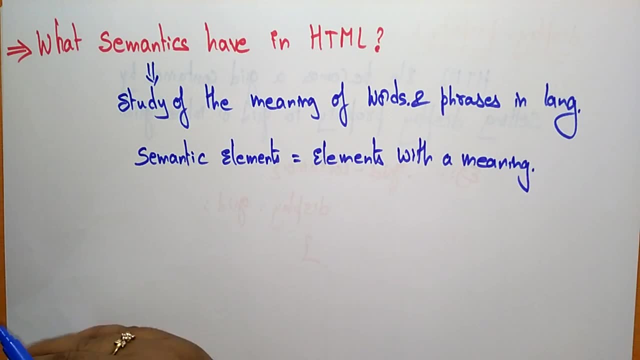 So it's semantic elements. So, whatever the HTML element that you are using, if that element is specifying the meaning of that usage, okay that you call it a semantic element. So, whatever the HTML element, there are rows of HTML. So, whatever that HTML element, there are rows of HTML. 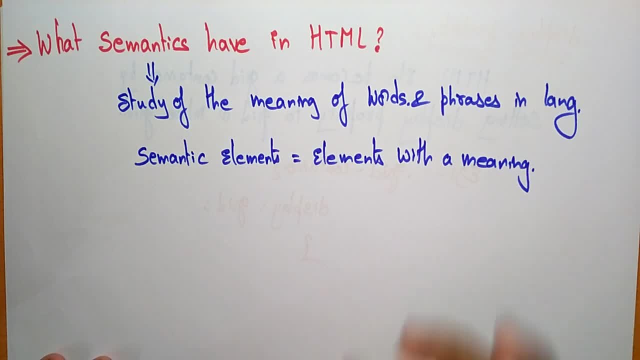 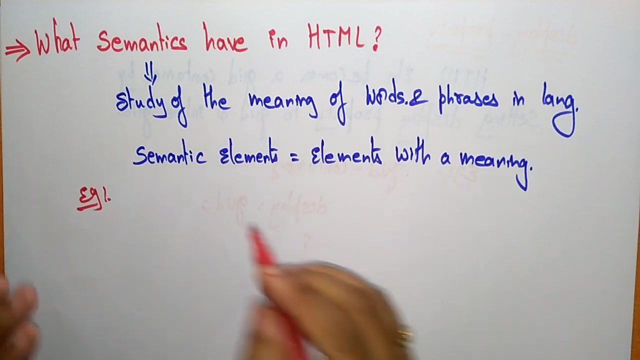 Some browsers that we use are described with semantic elements, offensive to секic elements. So we call it that semantic element. know what exactly the semantic element? uh, you just see the difference between non-semantic element and semantic elements in html. so in html you are having the both semantic and non-semantic. 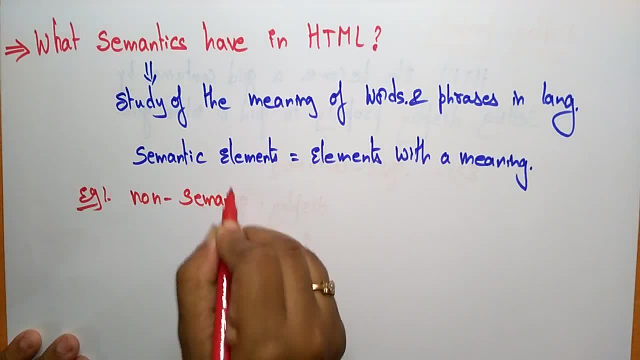 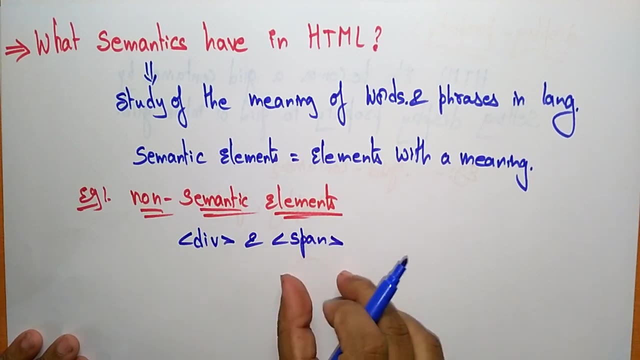 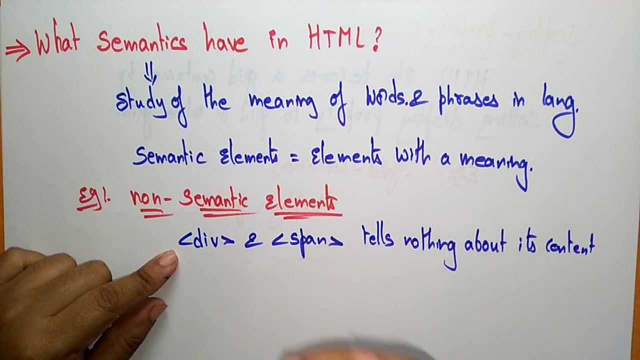 let's take the non semantic elements. so what are the non-semantic elements in html that we used? so those are div tag and span tag. so it tells nothing about its contents, tells nothing about its content, what it mean. so whatever you have written in using the div tag, so uh, in between, 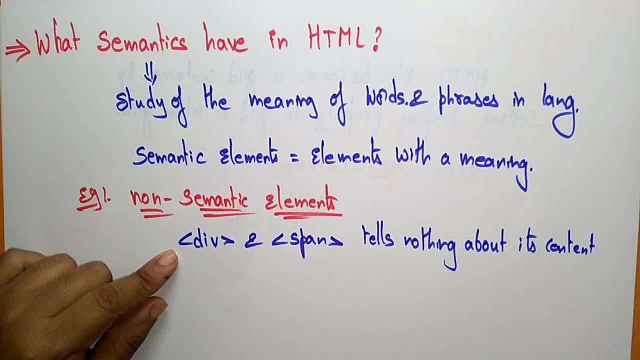 the div tag, some message will be there. so this div is not explaining what, uh, you're going to be inside. so this div is not explaining what you're going to be inside. so this div is not explaining what you are going to be explained in the same with the span, the row span, column span. so it 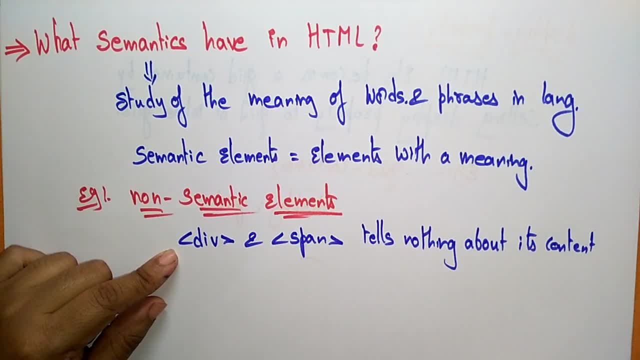 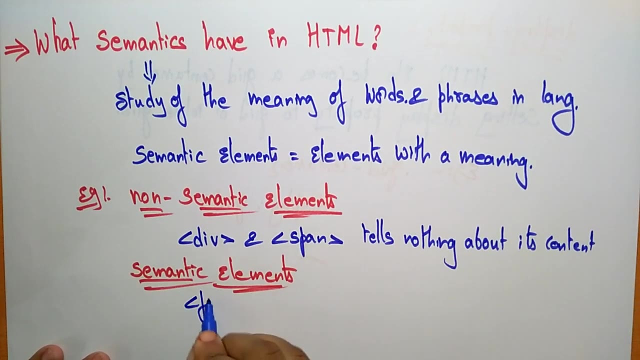 doesn't explain the meaning of what you are writing inside the span, so it tells nothing about its content. so then, what about the semantic elements? the semantic elements are nothing but form, table and article. the semantic elements are nothing but form, table and article. the semantic elements are nothing but form, table and article. 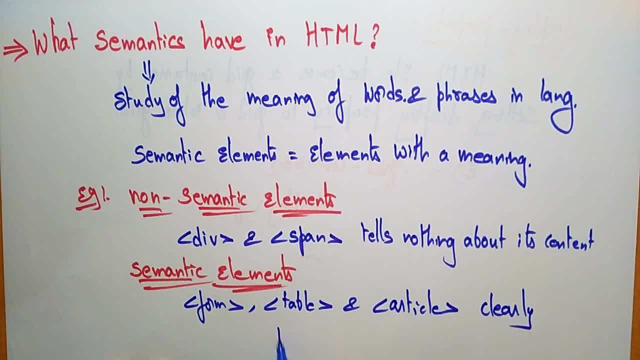 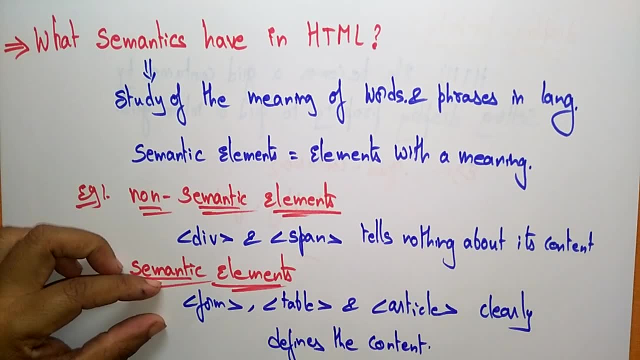 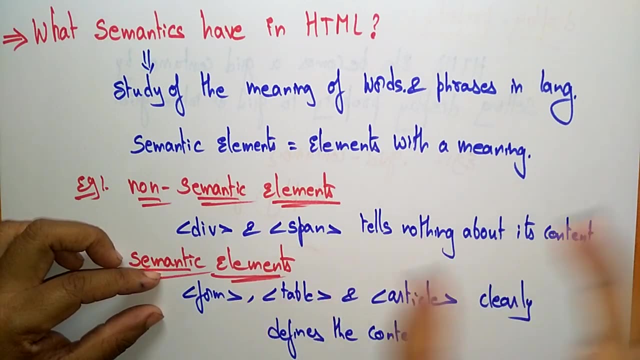 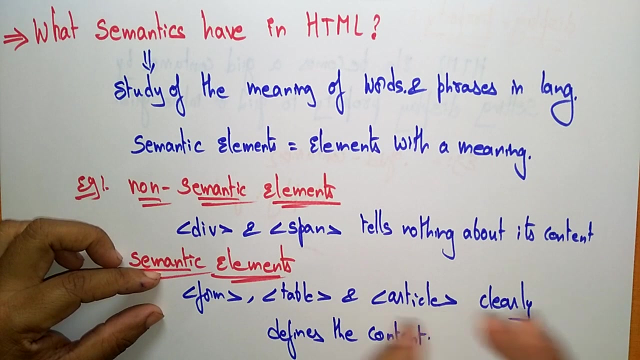 so clearly defines the content, clearly defines the content. so the form tag is itself, is going to display itself, is going to explain, so whatever the message that is there in the inside, the form tag that is going to be displayed on the screen and it is explaining that message. okay, that word, that is a form tag in the table also, it is whatever. 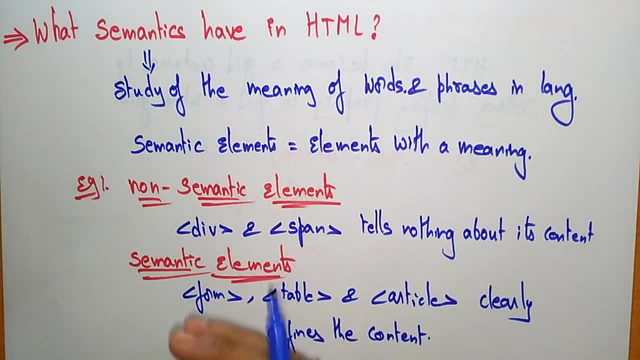 the data content that is there that is going to be arranged in a form that so that the user can understand and the browser can understand, like, in the same way, the article. so it is an independent element which is going to explain, showing whatever the message that you are returning in the article. 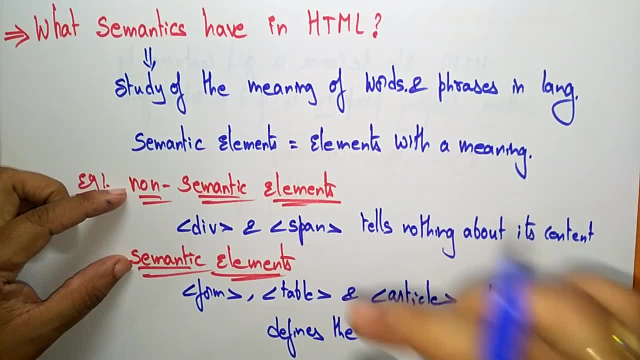 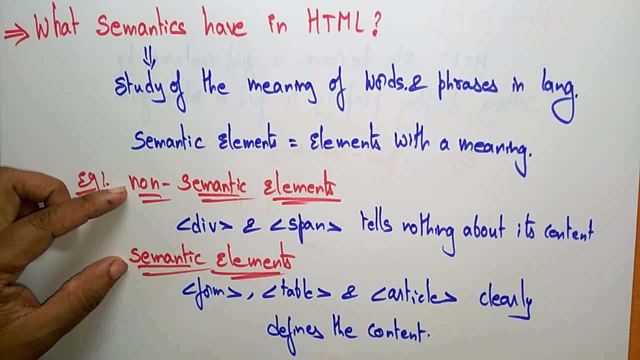 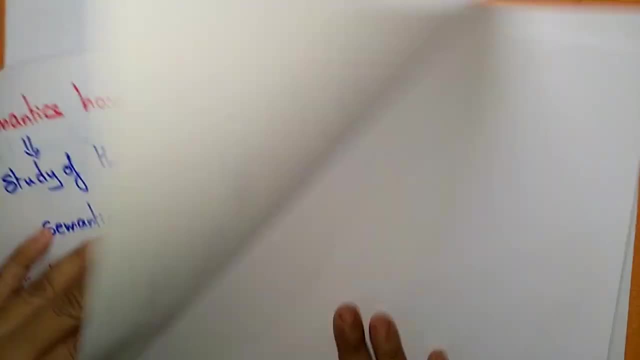 so this is the main difference between the non-semantic elements and the semantic elements. semantic elements, or can, defines the clearly defines the content, and whereas non-semantic elements tells nothing about its contents. let's see some of the new semantic elements that we used in html5. 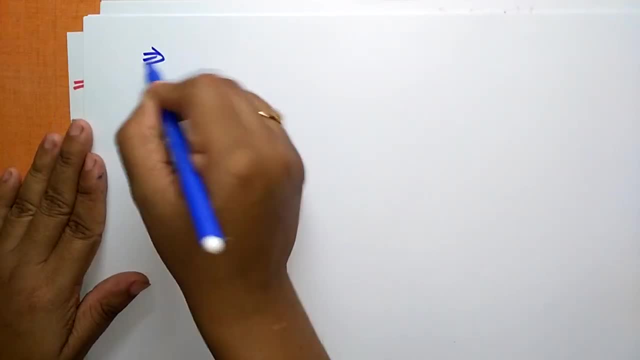 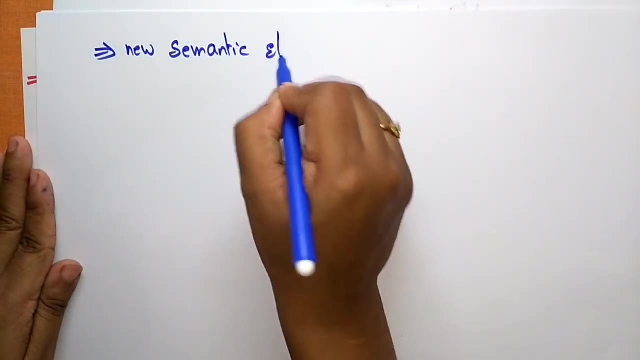 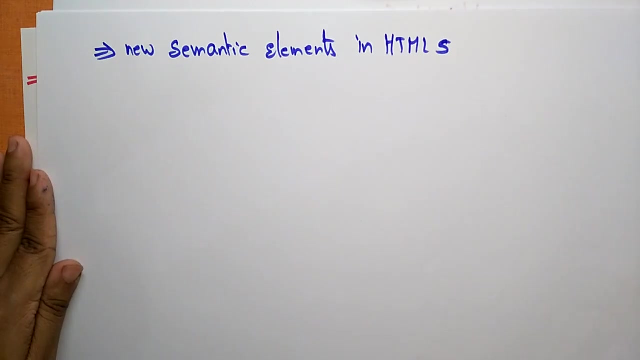 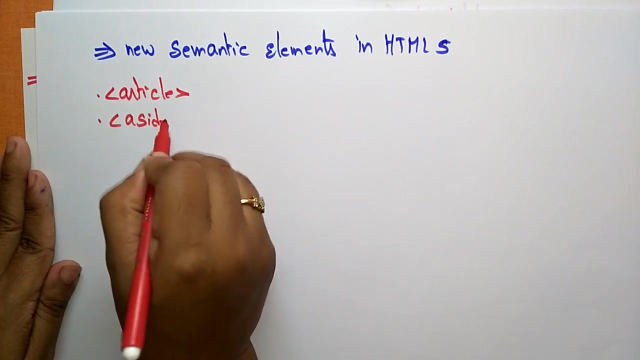 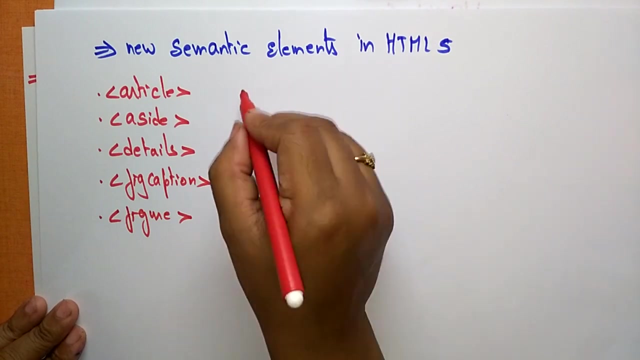 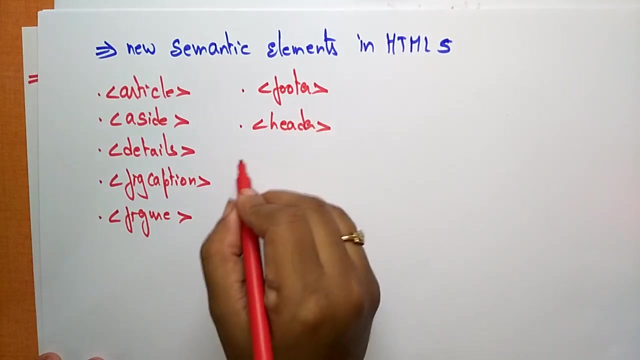 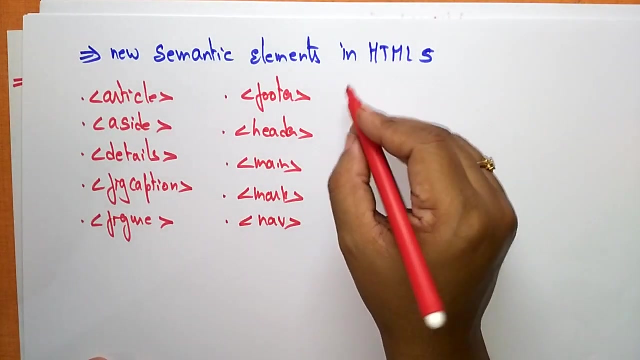 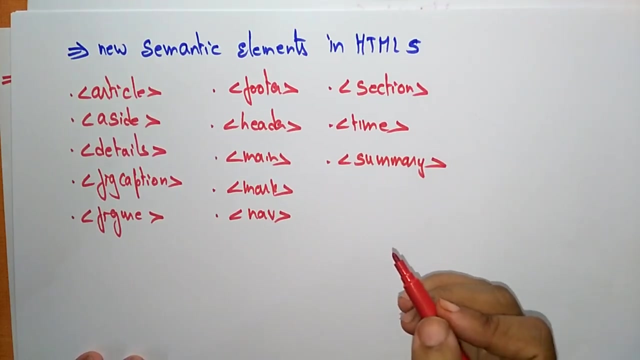 new semantic elements in html5. so what are the new semantic elements? article aside, details, figure, caption, figure- let's take a footer, header, main mark, navigate- so these are all elements. explains the: clearly defines the contents: event section, time summary. so these are all the different new semantic elements that we used in html5. so these just semantics. 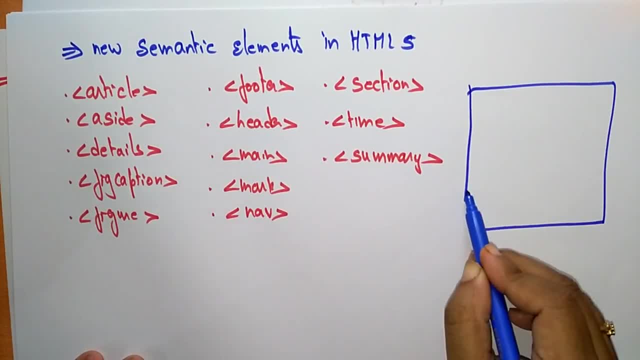 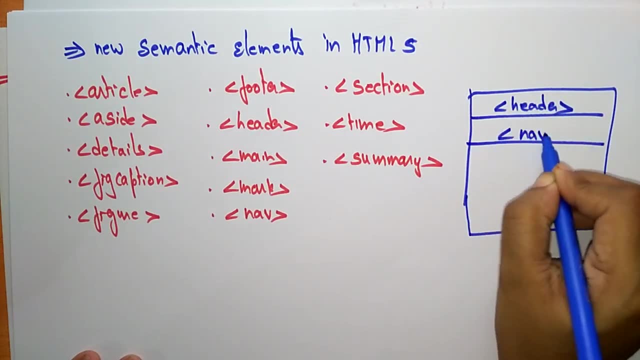 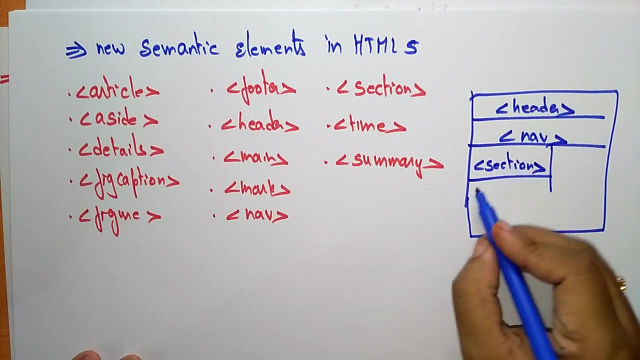 whatever the page that it's a web page consists of. so here in the web page, you are having the header, you're having the navigate button and you are having the section- it's a small section part- and even the articleiy- whatever the article you want to be displayed, and below that it is a footer.